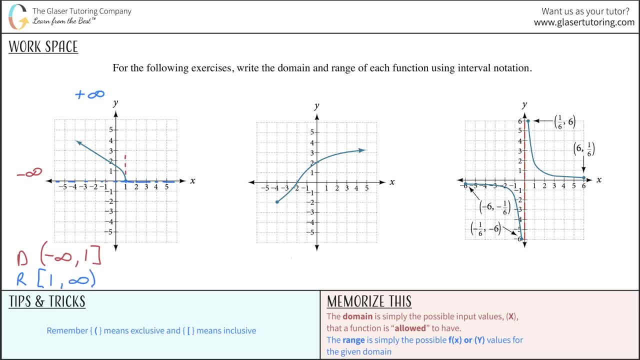 all the way to positive infinity and you can't include that because it's infinity. So this would be the domain and range and interval notation. Doing the next one should be just as simple, right? Leftmost point of the graph is: x is equal to 4 and it includes it. The graph is: 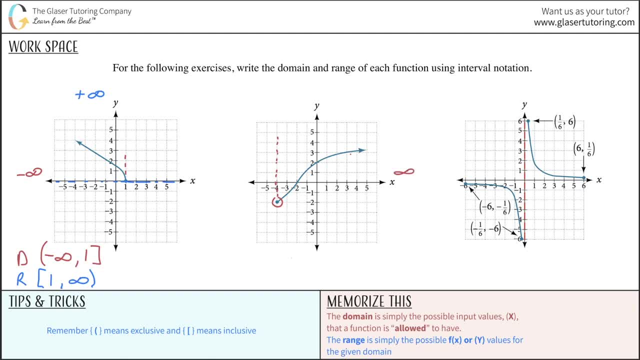 going to go on forever. So in the x direction it goes on off into infinity. So, thinking about the domain of this, it's going to include negative 4 and it's going to go all the way out to positive infinity, exclusive of it. The range now is going to be similarly, you now. 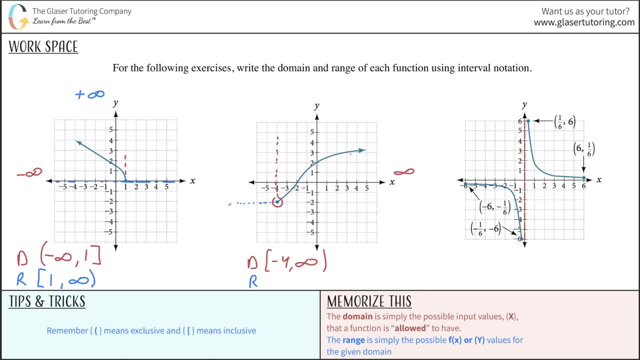 look at drawing horizontal lines right. Right, the lowest y value here is going to be negative 2, inclusive of it, because the circle here is filled in And now it looks like- and this is a little tricky, but if you zoom in enough it's going out like this: okay, The graph does have a slope to it. 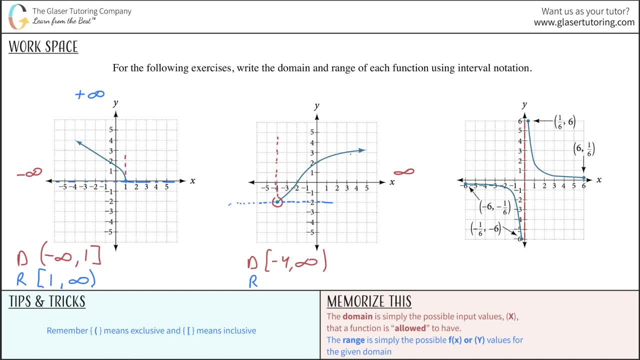 and therefore this arrow means it's going to go on and on forever. So it's going to go all the way up eventually to positive infinity in the y direction. okay, So the lowest y value is negative 2,, exclusive of it. so that's why the bracket all the way up to then positive infinity, exclusive. 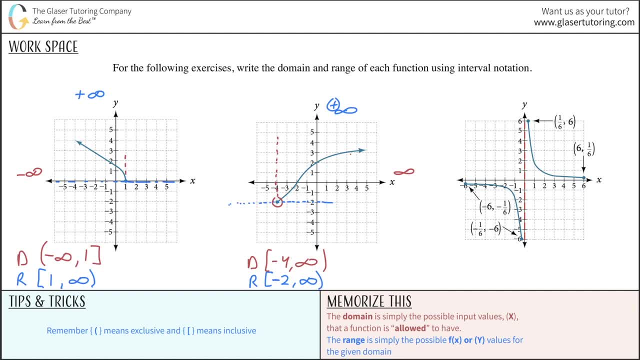 of it. So this is the set for domain and range. Last but not least, there's numbers all over the place, So this one we have to deal with in two pieces. okay, There's two parts of the graph: there's one part over here and then there is another part over here. First, let's look at this. 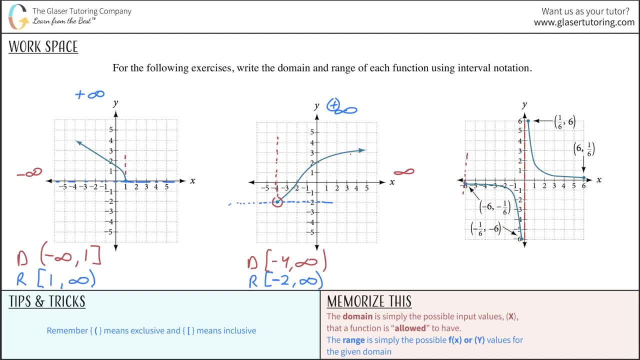 particular piece, The leftmost point of the graph is going to be. x is equal to negative 6. So this is the lowest point of the domain Then. so we know that and it's inclusive. It's tough to see, but that is a filled in. 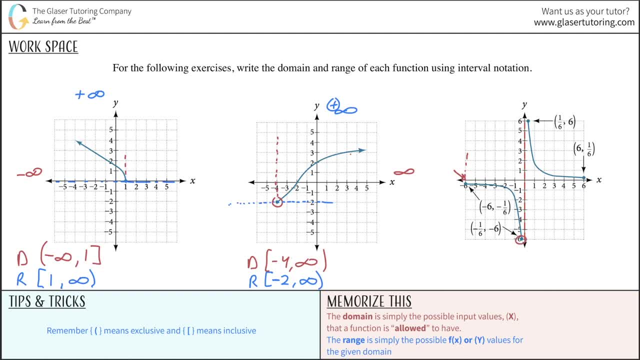 circle. And then it tells us now, at this particular location, it gives us the ordered pair here that defines this filled in point. What's the x value of this point here? Well, it's negative. 1, sixth right, That is how coordinates are given: x, comma y. So we know now for this particular piece. 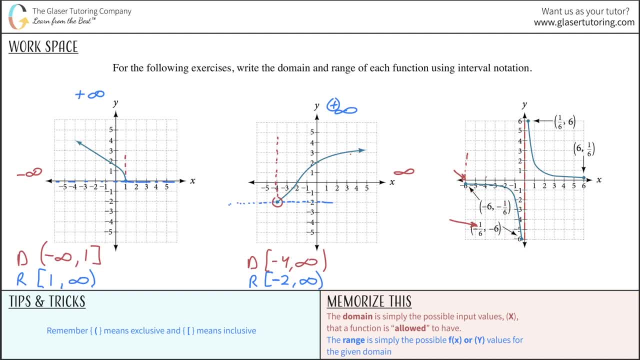 of the graph. we do indeed know that the domain here for that part is going to be negative 6, comma inclusive of it, all the way to negative 1, sixth inclusive of it. So that takes care of this first half, all right, So now. 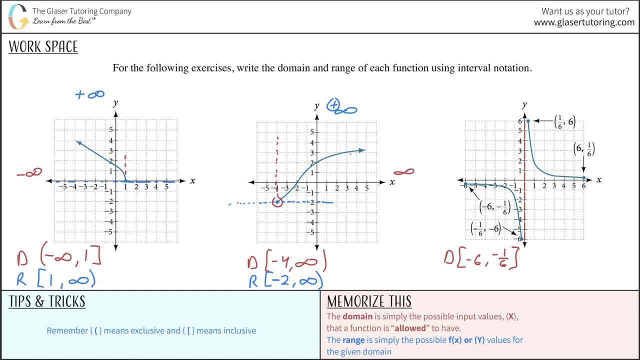 let me just erase these arrows just to make it a little cleaner. And now we realize that we got to do the second half. okay. So now notice the graph on the second part. the leftmost portion of it goes all the way out to 1 sixth. okay, Inclusive of it, because it's filled in. 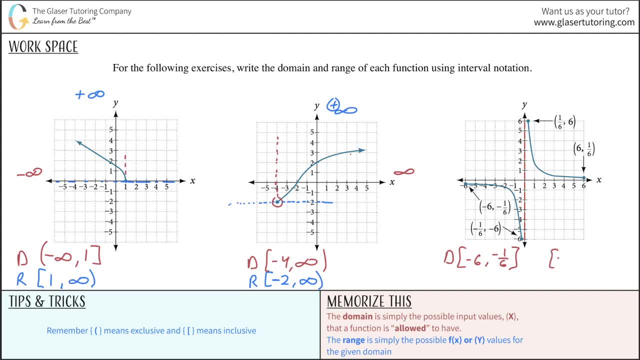 So now I'm going to write another bracket, 1, sixth, now, inclusive of it, And it's going to go all the way on out in the positive x direction, all the way out to 6, because that's what it told me, Inclusive of it, because the circle's filled in Now, since you have two components, that the 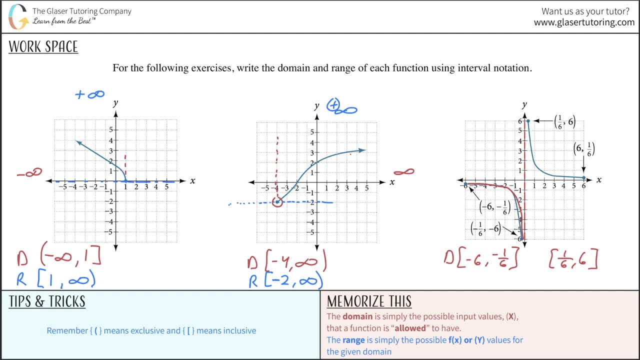 x value could have been at any point on this graph, or that's the key word, or any point on this graph. anytime you hear the word or it is considered inclusive of it. So now I'm going to try to close this right now. Okay, I'm going to go into my 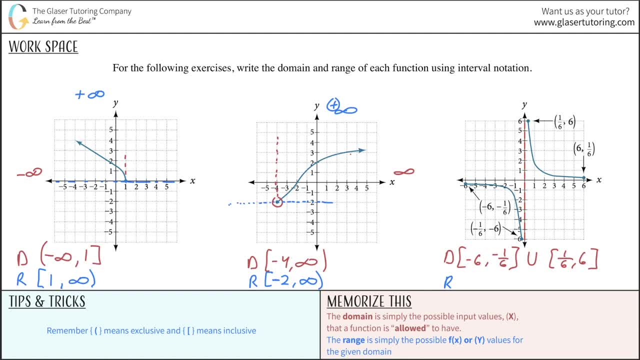 building, and this is going to look at this there at the at the 2nd half, and I'm going to put, and it will say 1- most into 1, because this circle is now going to be 0. So, literally, at the end, this circle will be 1- 6th. but you can actually still keep that symbol if you were going to write another option down in the data tab. So the plus 2和. so you'll notice here that's 1, 1, sixth the upper half, and then you're. actually 2, 2 stuff inside this, that circle, and then you actually need to have a reason to cross it out. as a surface, You could write an X, Yes, and forgiveness becomes 1 minus 1.. So now all I have to do isлонat. 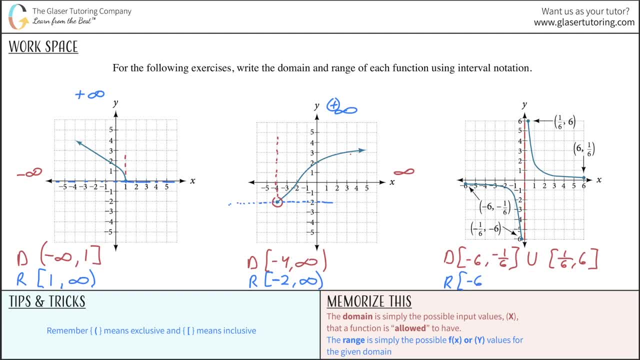 leftmost portion. it's going to go inclusive now of negative six, all the way out to negative one, sixth inclusive, Or we could have been over here, right. So, union, I'm going to use another bracket because I know all of these dots are filled in, So I know they're all going to be inclusive.